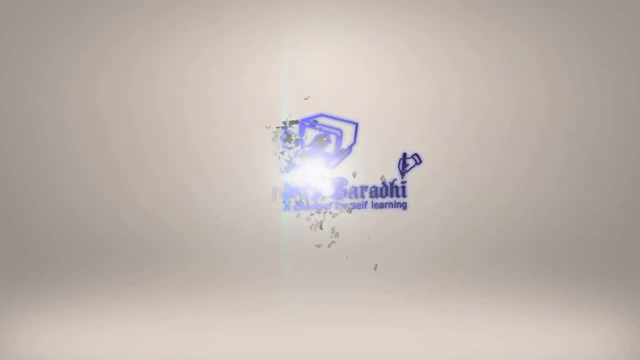 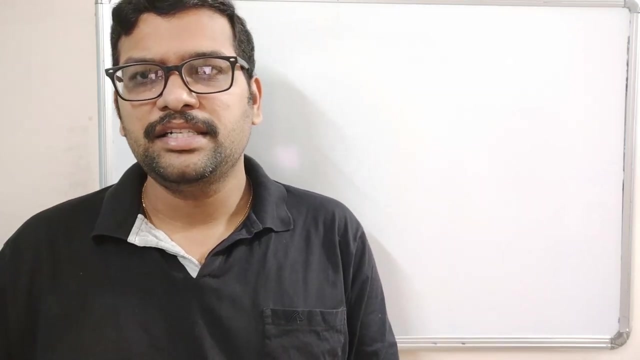 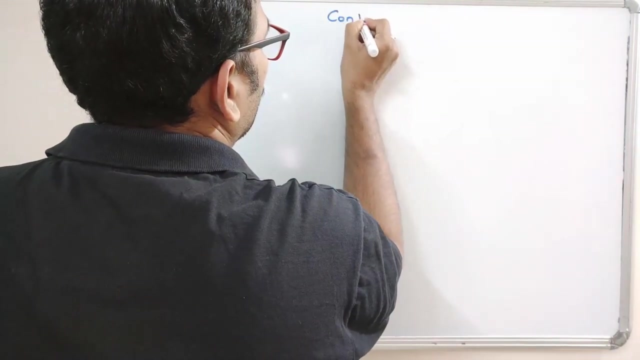 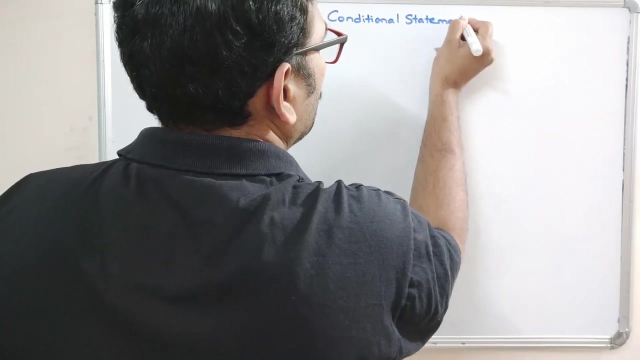 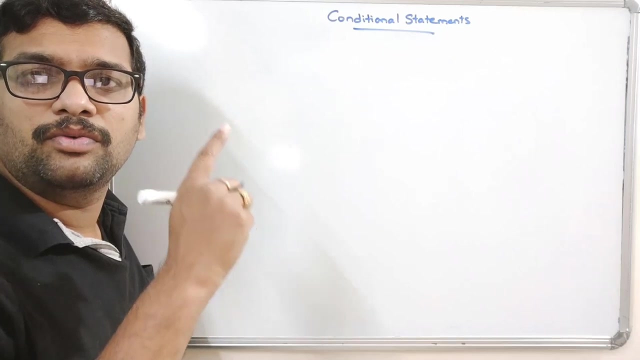 Hello friends, welcome back to our channel. So in today's session we will discuss about the conditional statements in JavaScript. So here the name itself indicates based upon the result of the condition. So we have to decide which block should be executed. So 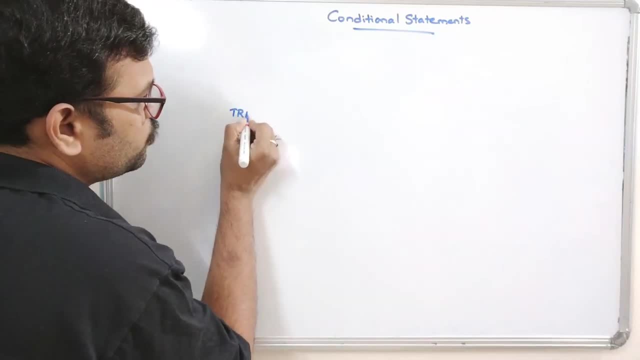 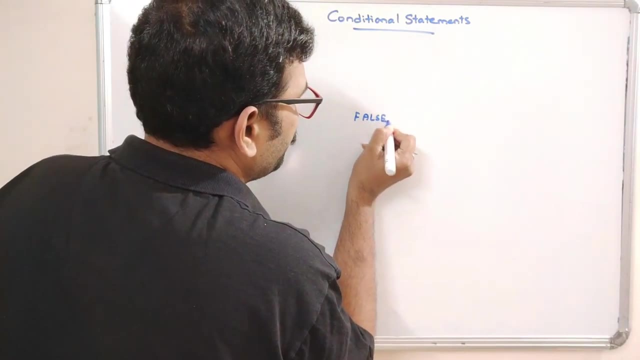 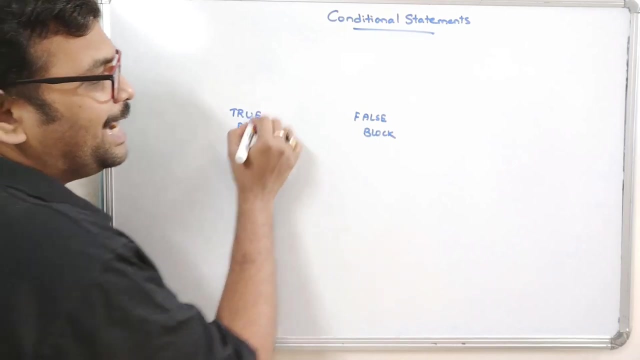 here there will be two blocks of code. that is true block and this is a false block. So only one block of code will be executed, but not both, So that decision will be taken by the condition, the result of the condition, So based upon. 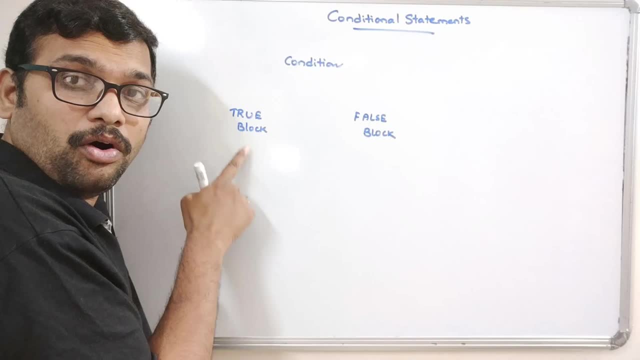 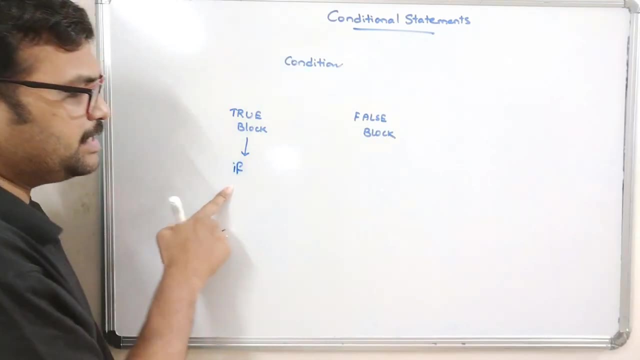 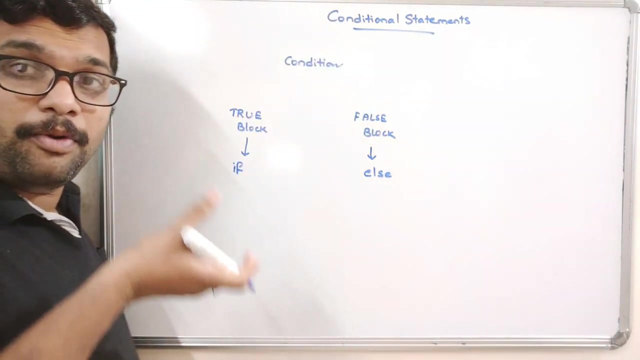 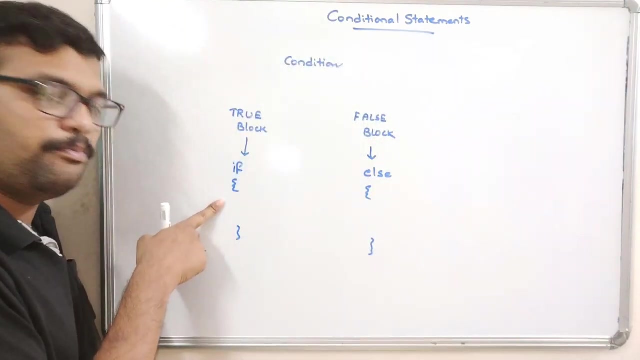 the result of condition, either true block will be executed or false block will be executed. So this true block will be written as a if-so And this false block will be written as a else statement. So we will write some block of codes in if and else. So this if block is represented as a true, else is represented. 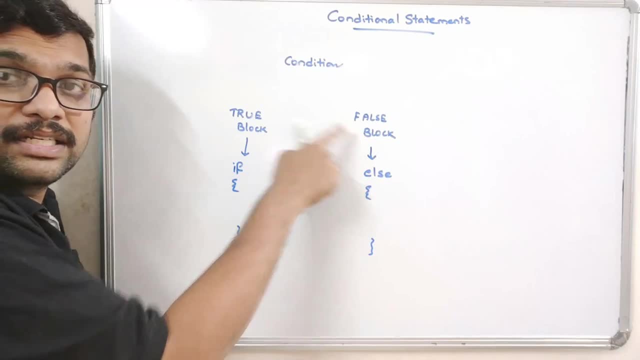 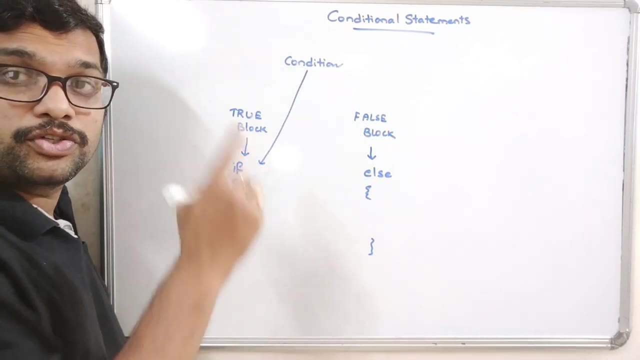 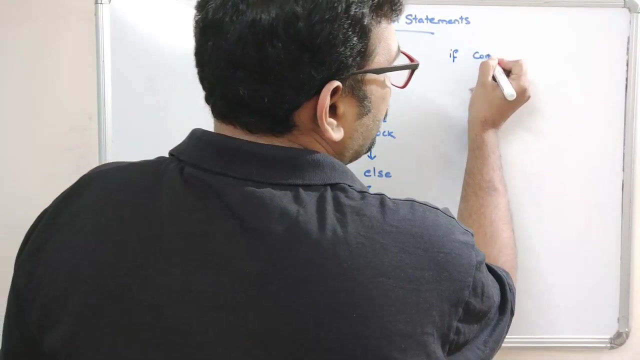 as a false. And here the question is where we have to write the condition. So this condition should be written in true block itself. So we should not write any condition in true block. So here the syntax will be: if, followed by the condition, followed by the condition. 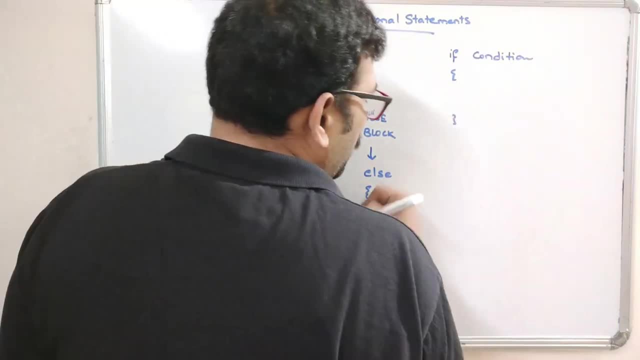 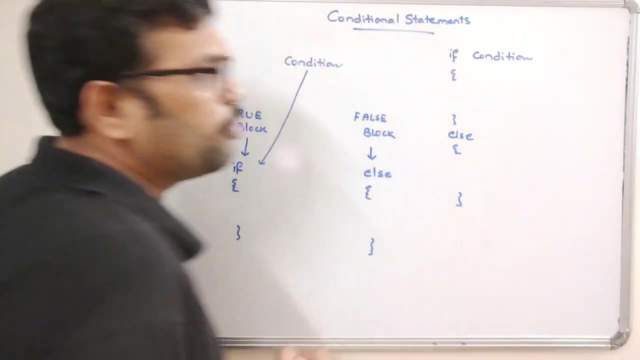 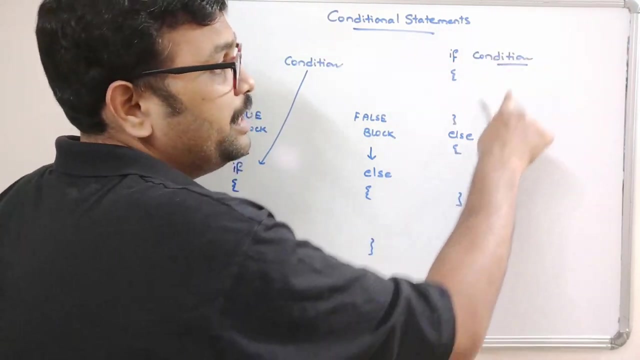 and write down the block. And if you want to write the false block also, you have to go with the keyword else and write the code here. So based upon the condition, if it is true, this block will be executed and this will be ignored If the condition is false. 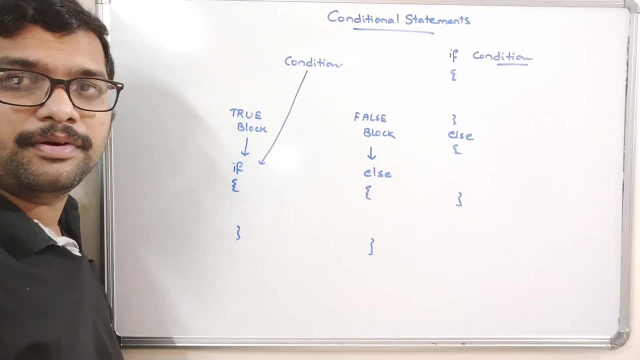 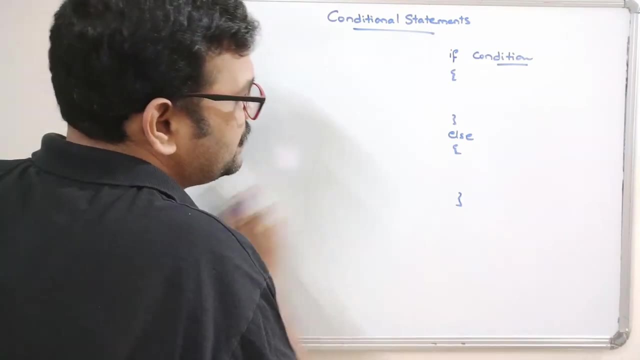 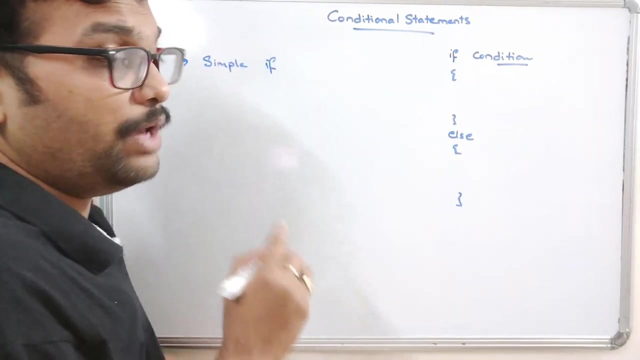 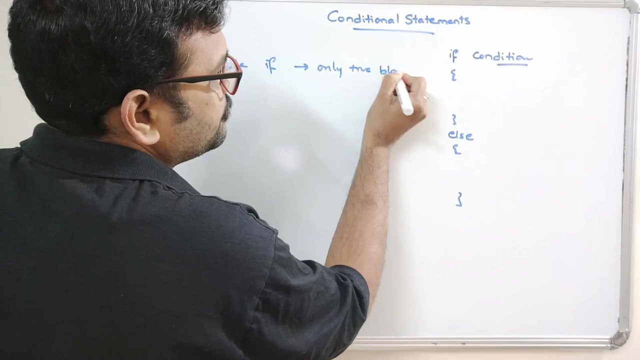 this block will be ignored. This block will be executed Right. So mainly in this session we are going to discuss about the three types of conditional statements. One is simple, if simple, if where we will write only true block, So only true block will be written here, Only true block will. 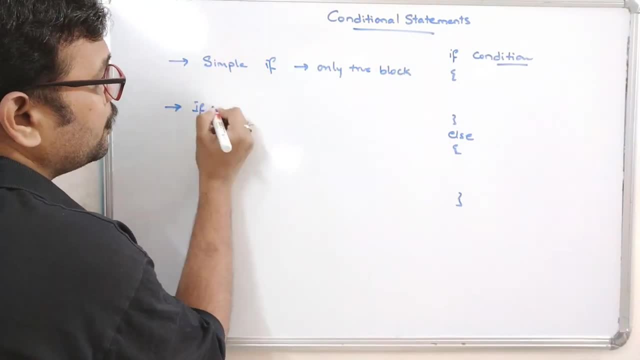 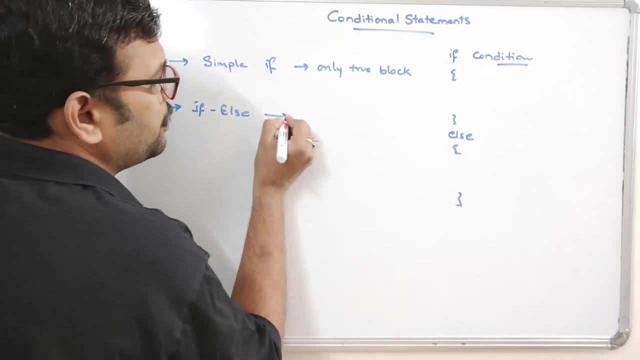 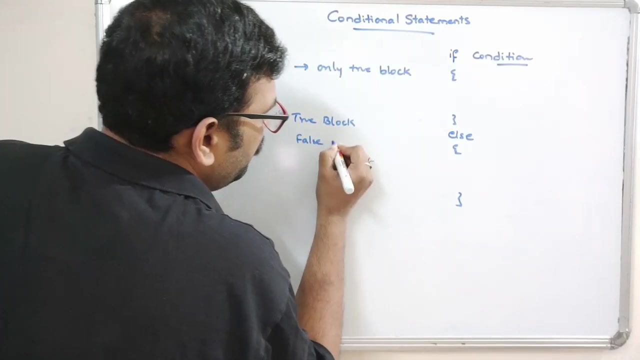 be written, And the next one is if-else. If-else means both the true block and the false block will be executed. So true block and the false block, both will be implemented here, But it executes only one And the next. 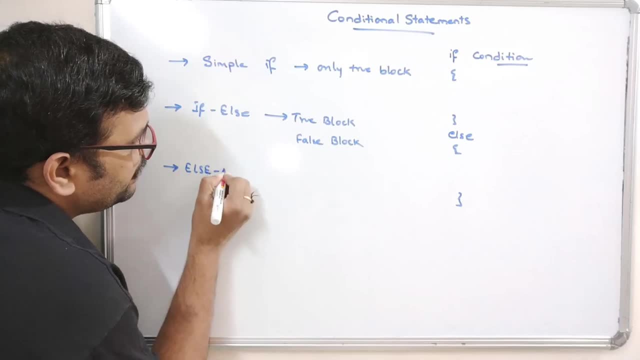 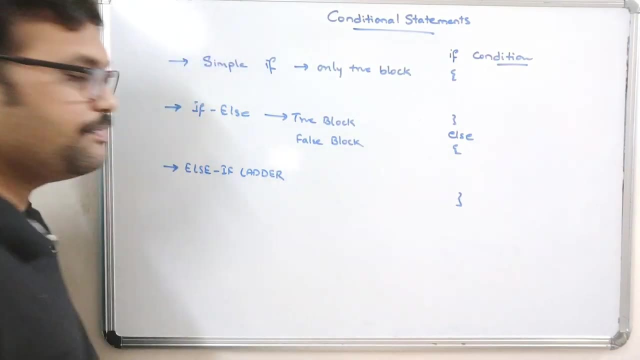 one else-if ladder, Else-if ladder, That means if-else, if-else, if-else, if-else, if-else, if-else. So if the condition fails, if you again want to check one more condition, 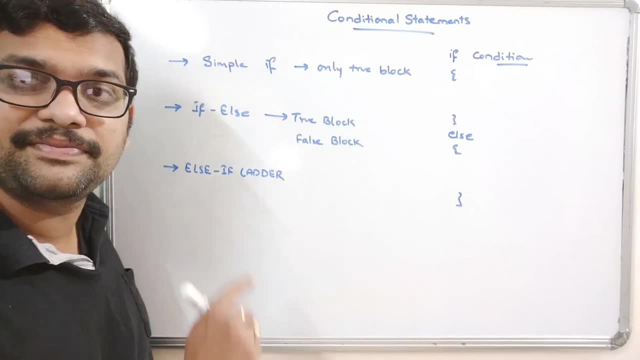 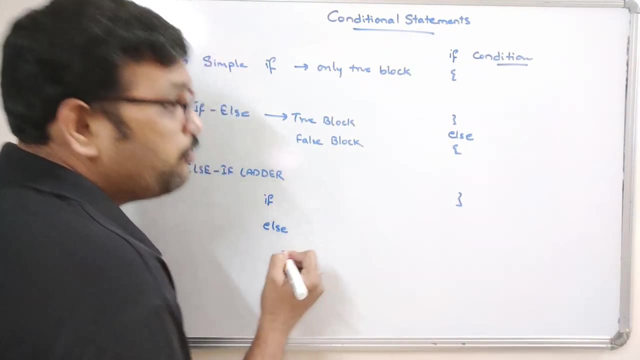 that means, in order to check more than one condition, we will go with this else-if ladder. So here we will write some if-true block. okay, then else-if and what we have just now. we have discussed about this one, so we have to write the condition only in the true. 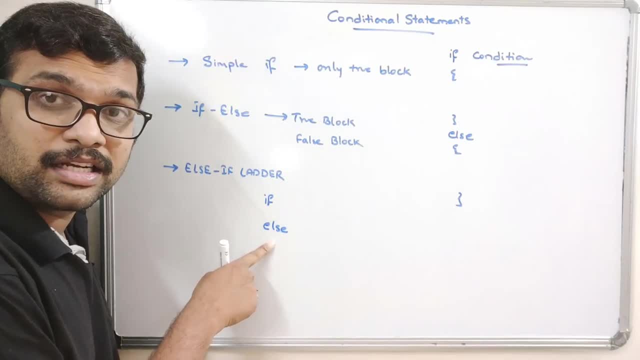 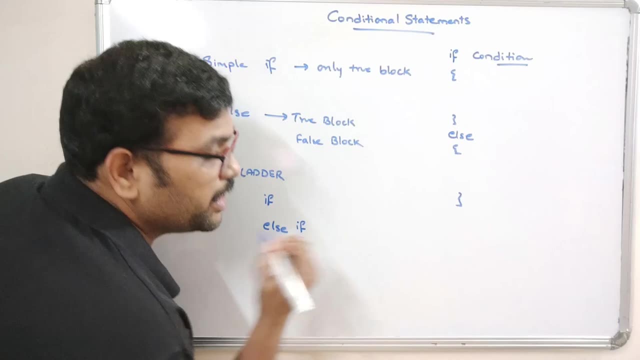 block. So we should not write the condition else in that to the false block. So if we want to check one more condition in the false block, you cannot write the condition in the here, just include if, and followed by the condition and if you again. this condition fails again if you. 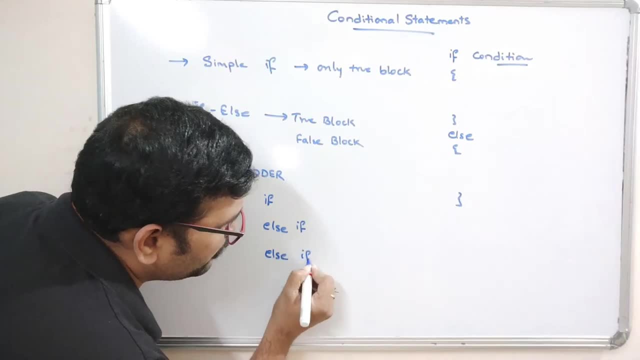 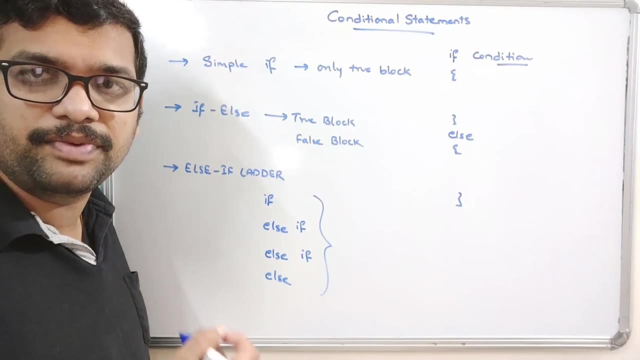 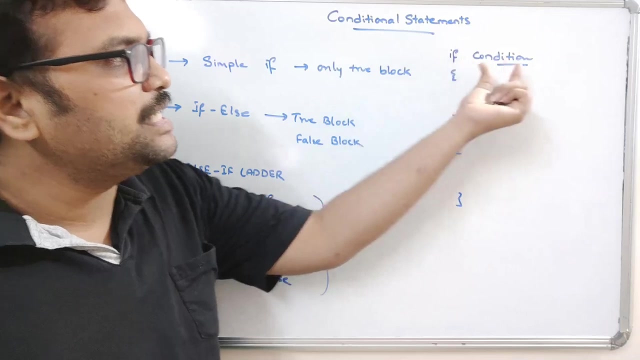 want to check one more condition, go with the another: else, if and else. so this is a else- if ladder. so we can check multiple conditions. we can check multiple conditions, right. so one thing: based upon the result of the condition, we are deciding which block should be executed. 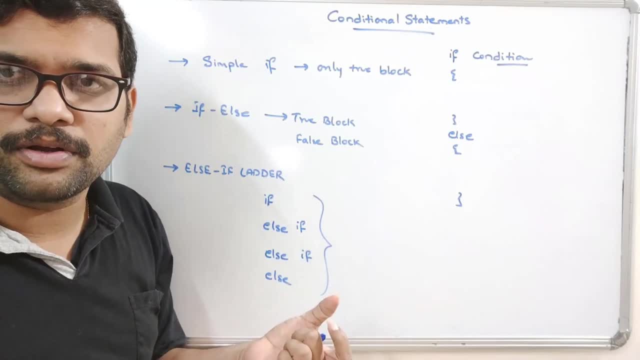 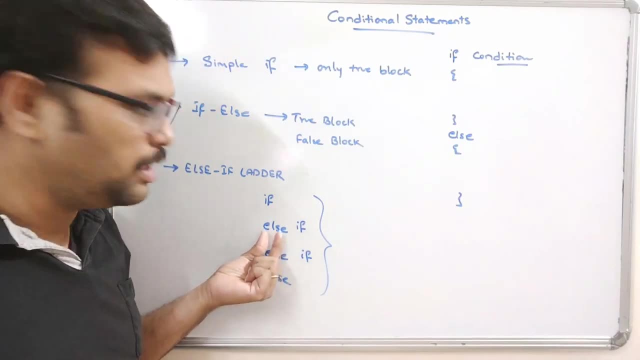 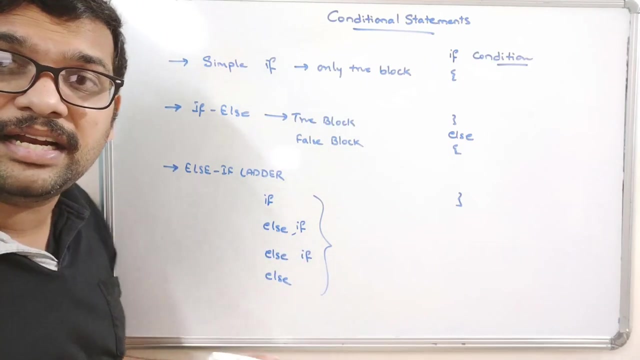 so either true or the false block. so if you want to check more than one condition, just include the true block at the false block. that so that that forms the else, if else. if so, there must be space in between else and if right. so this should be implemented at this. all this statement should. 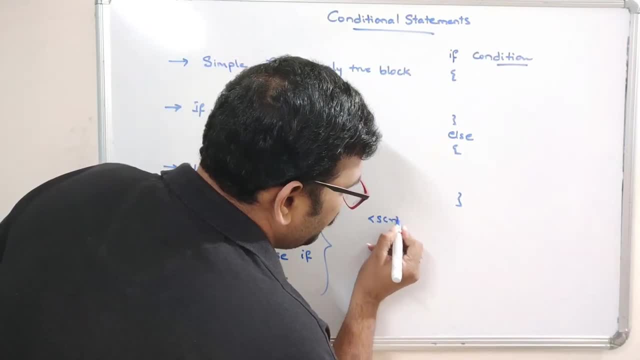 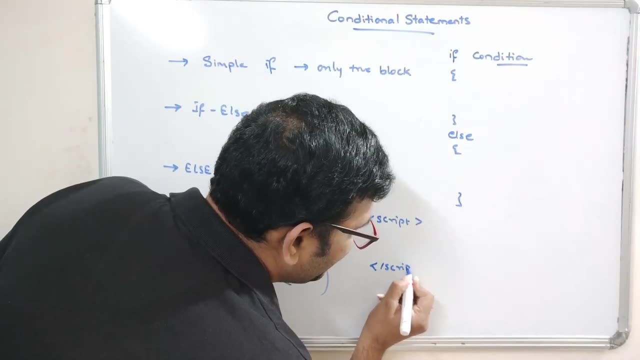 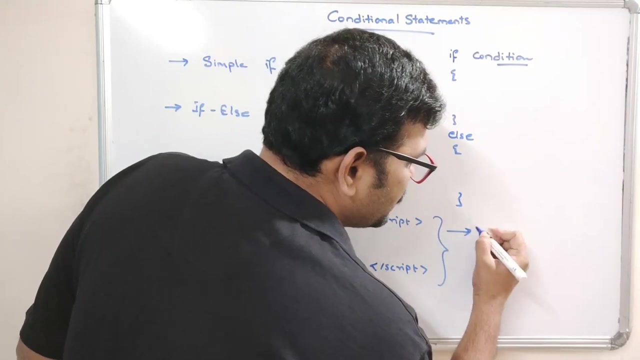 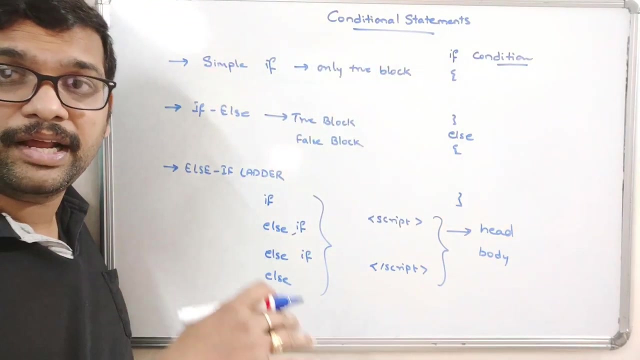 be implemented in script script tag. okay, all these are the JavaScript, so we have to include all these things inside the script. and where we have to write the script, as we have discussed in the previous sessions, we can include this script in either head or a body, so cannot anywhere. in the head we can write the script, or in the body itself we can. 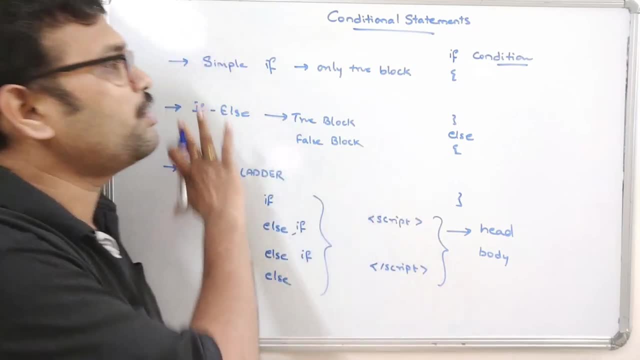 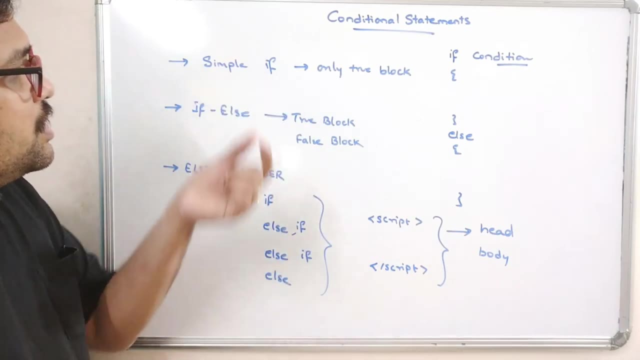 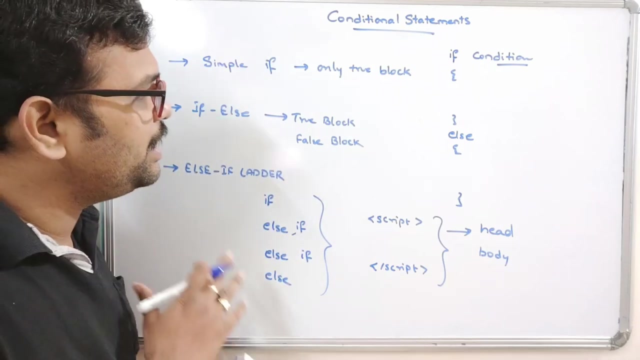 write the script, so no problem. so inside the script we have to write all these things, we have to implement all these things, right? so this is the basic thing, and in this session we are going to discuss about this simple if, if else and else, if later. so i will demonstrate all these three. 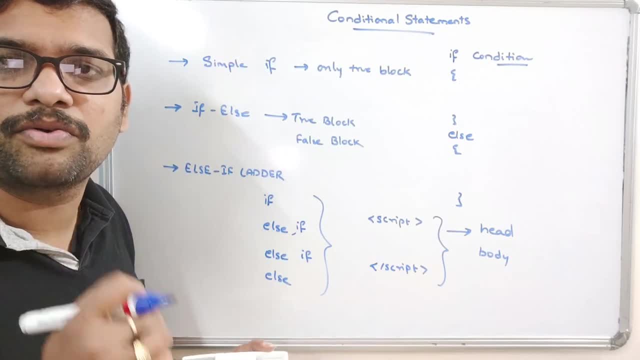 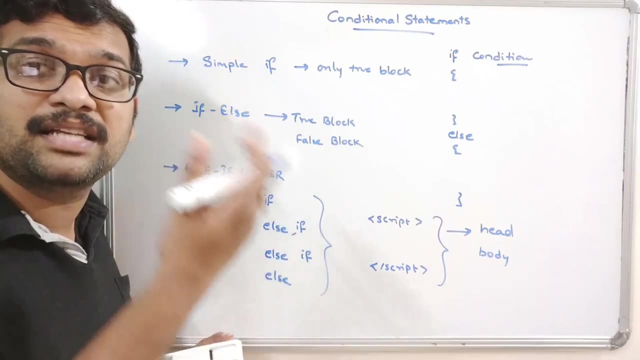 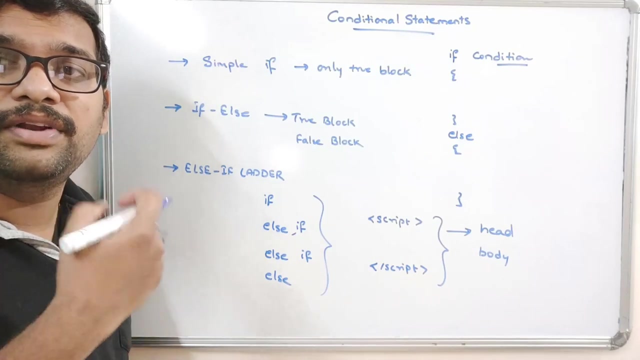 conditional statements by executing a small html code, so we'll see the script where we are writing these conditional statements as well, as we will apply some style sheets- okay, some styles- to the existing tags as well as we have. we will see the output statements. so these output statements also. 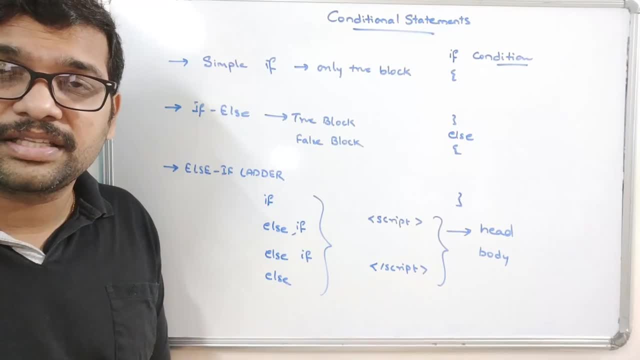 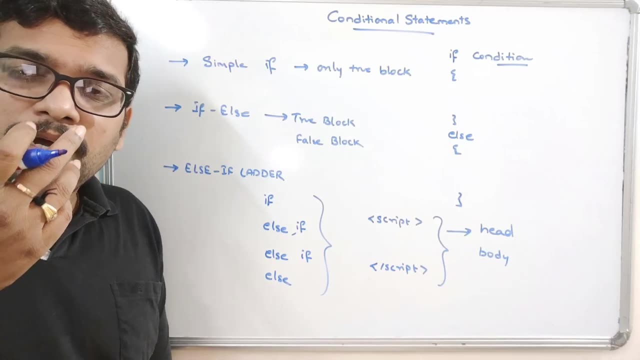 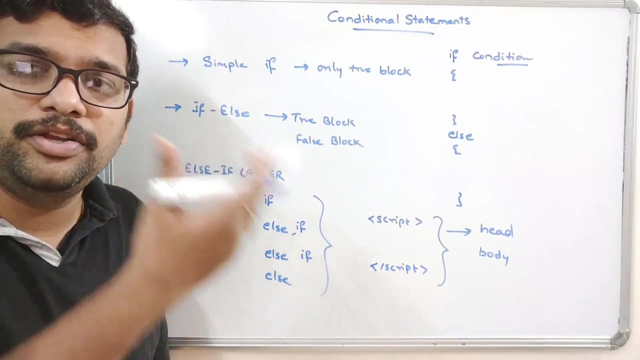 been covered in the previous sessions. that is three, three cases, three ways. we can represent the output on the javascript by using the document dot write ln or document dot. i mean inner html or window dot alert the three cases we can display the output. so we'll use any one among these three and we'll demonstrate these. 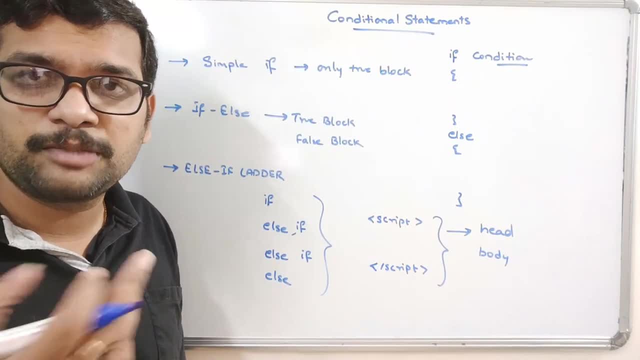 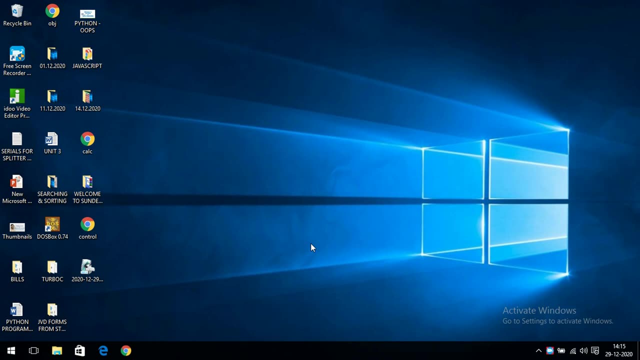 conditional statements by executing a small code. so let's move on to the system. hello friends. so we have seen the syntax for the conditional statements in javascript, that is simply if else and else if later. so in order to demonstrate all these things just, we'll write some code. 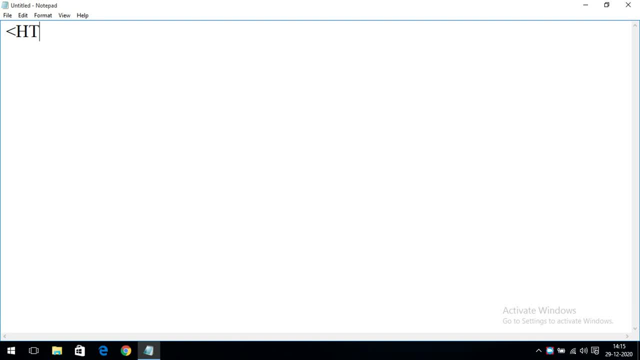 and i will explain you. so first of all, let us start this with the html. so in between the html tag we have to include all these things, and inside the body, first we'll write one form, yeah, and here we'll create one form, just we'll give one text box to read the input. so for creating. 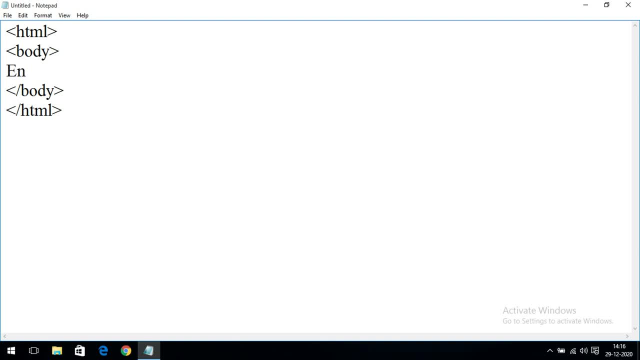 the text box. i am taking this one: enter age. okay, so enter the age. so we are finding whether the person is eligible for both or not. so here i am just giving some text box. input type is equal to text. and i am also giving giving some id is equal to t1 right. Then after that I am just giving some button. I 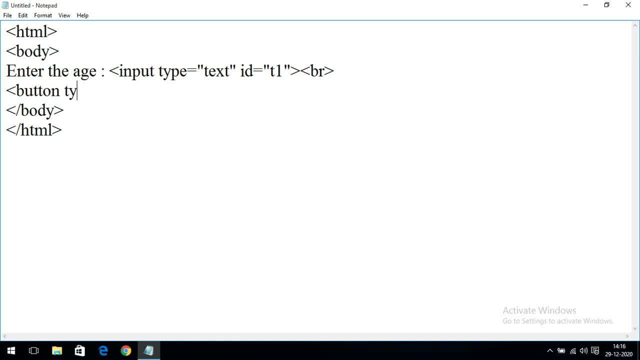 am creating some button here, So button type is equal to button and here on click. So whenever it was clicked some trigger should be done on click is equal to. I am giving some function, age and closing here. submit or verify. we will go with the verify. I am taking some. 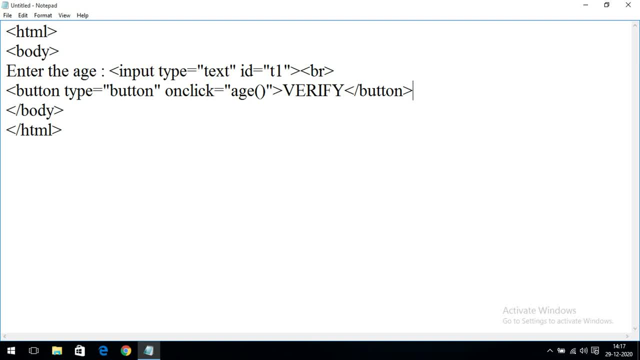 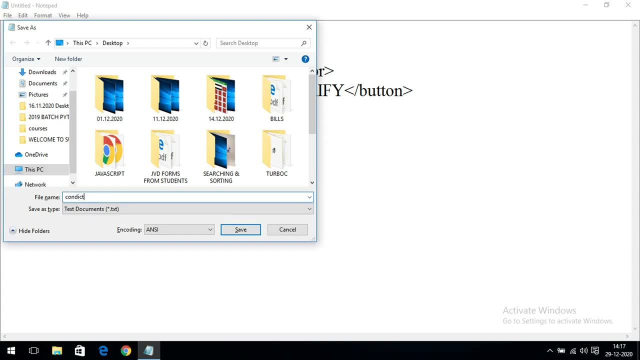 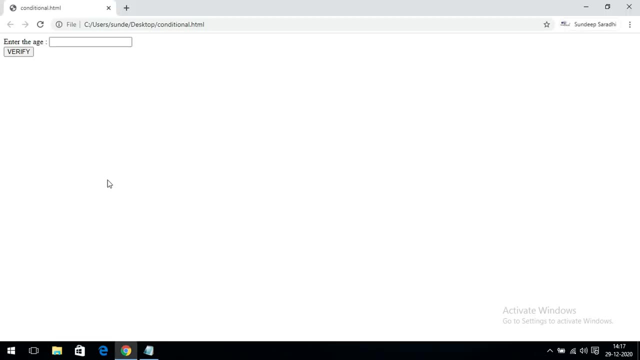 button. I am closing the button, So I will save this one and we will check whether the form was created. So conditionalhtml. So move with the desktop. So here you can find conditional, So you can observe here. 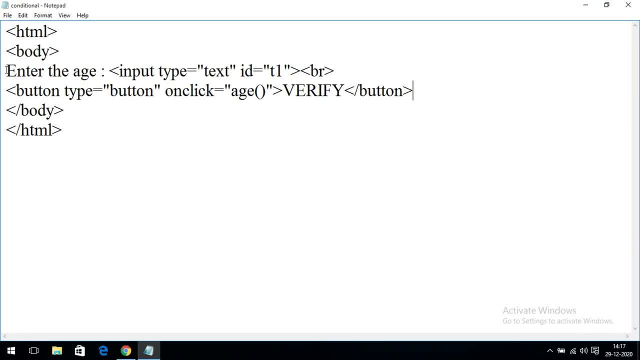 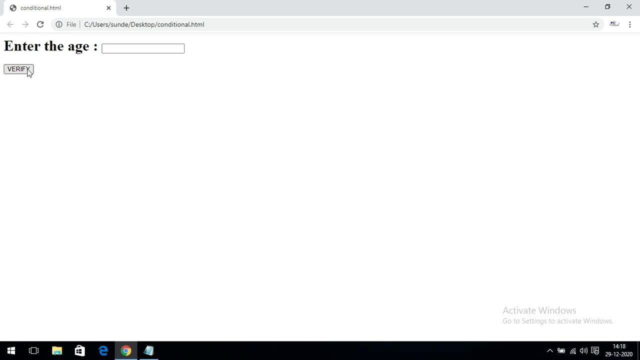 enter the age and verify. ok, enter the age and verify and we will give some h1, because text is very small. So if you give this h1, automatically the text will be picked up. So here you are. you are supposed to give the age and we have to verify whether the 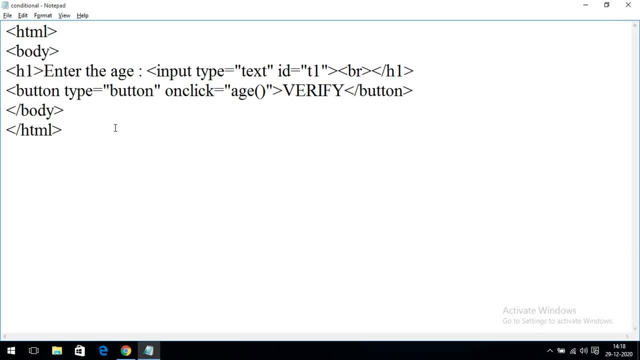 age is. I mean the person is eligible for vote or not. Now, after clicking on this age, we are giving some age function. So we have to write the function in script, because that is a JavaScript. So I am just writing the thing in script tag in between the script. 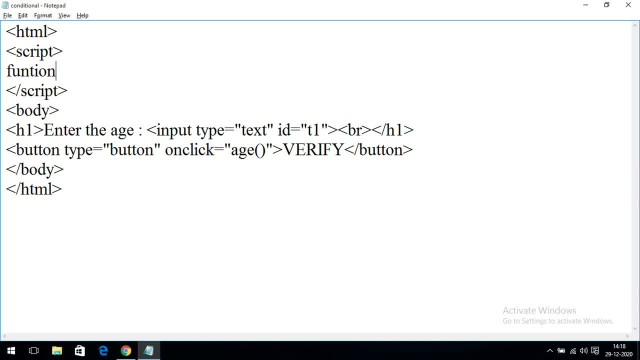 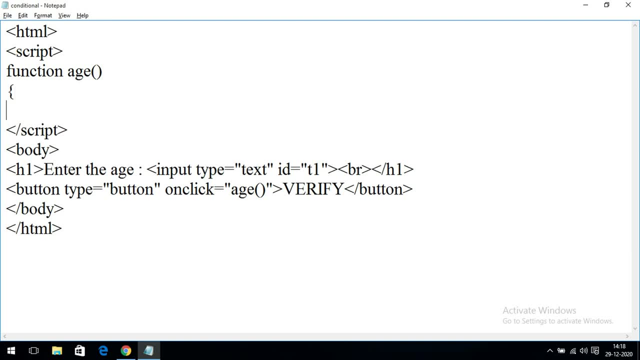 tag. So here we have to write: So function, So function, So if h, so what we have to check. I have to check whether he is eligible. That means we have to check if condition So documentGetElementById- grater than or equal to 18.. 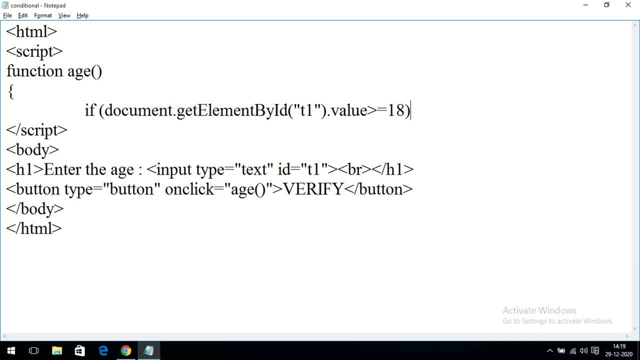 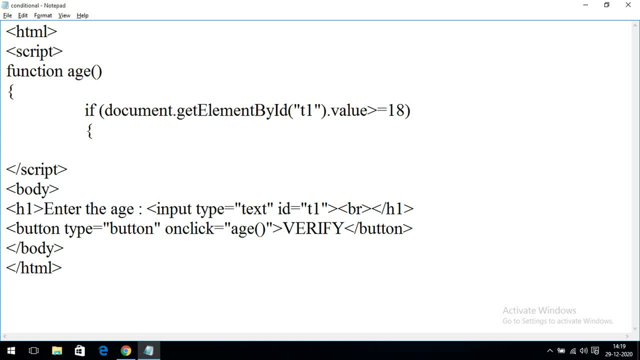 If the value is greater than or equal to 18, obviously the person is eligible for vote. So where we have to write, we have to display at some place, Okay, Or simply we can write some windowalert, windowalert eligible for vote. 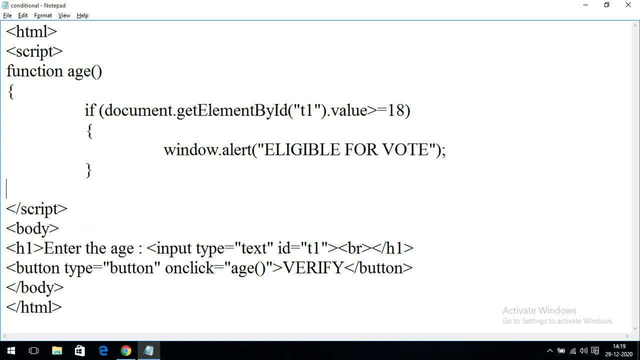 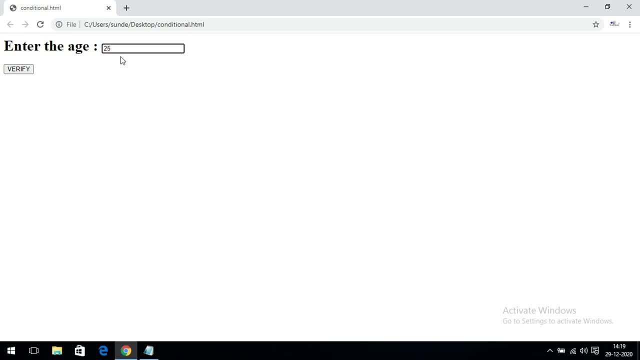 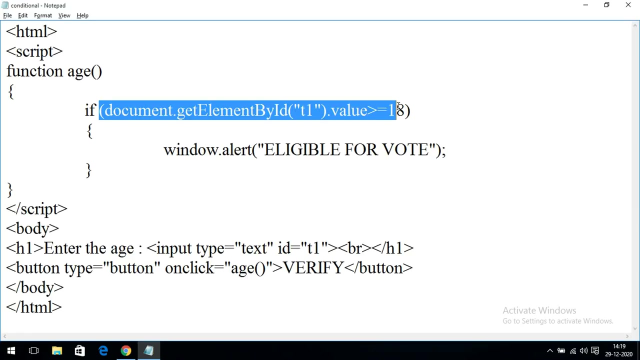 Okay, This is a small, simple if statement. Simple if statement. Okay, So just here, you can give some 25 and verify will get eligible for vote, Right, If you go with some 15,? if you click on verify, it does not give anything else, Right, Because we are writing only the true statement. We are writing only for the true condition. 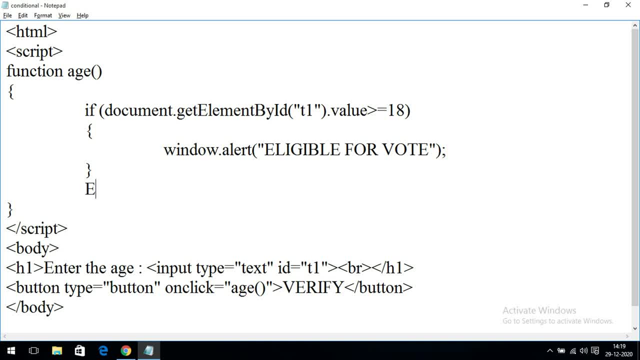 Okay, If it is false, then we have to display at some place, So go with the else part. Okay, That is called a simple if and else. So here we can write. So windowalert not eligible for vote. 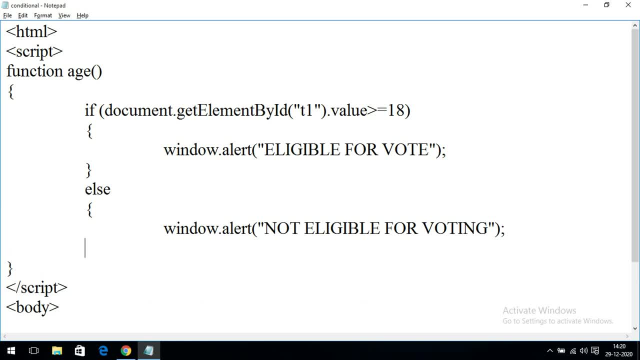 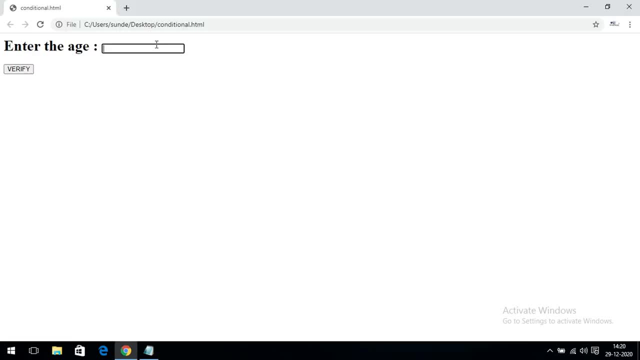 Right. So this is the else part I have written. Now you can observe we will get both the results If you press. if you give any age greater than 18,, automatically we will get eligible for voting Okay, And if you give any age below 18, we will get not eligible for voting Right. So this is one way And if you want to display the same thing, 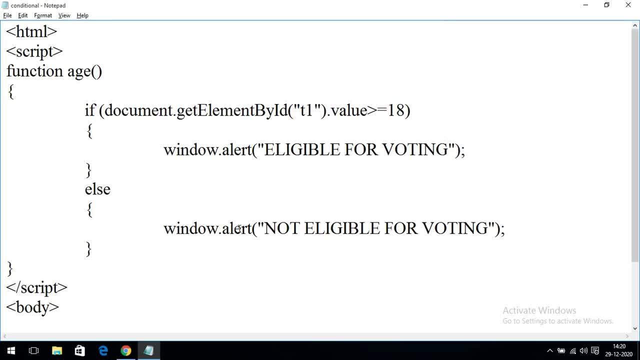 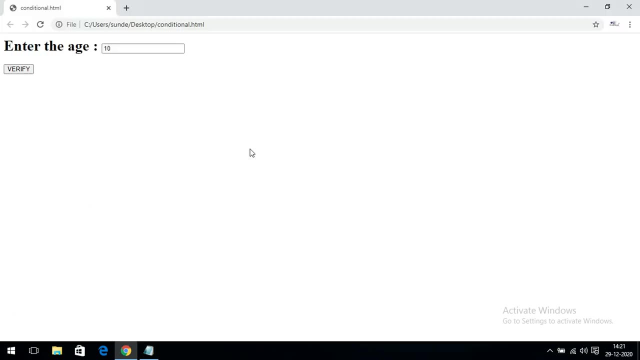 In the document itself without using the windowalert. we are having one more thing called documentwriteln, or we can also go with the inner HTML. Okay, Okay, Yeah, You can observe here. eligible for voting, Right. So otherwise we can also give some. 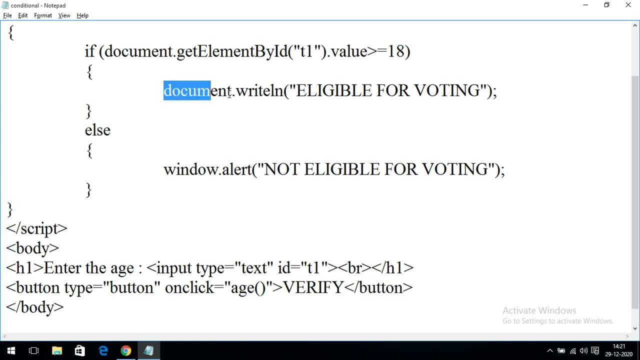 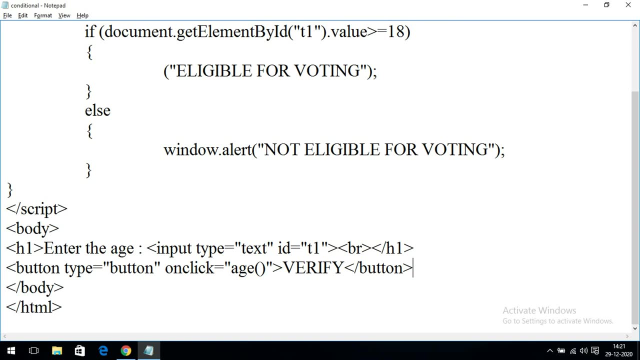 In our HTML. Okay, So anyway, we can write any. we can use any output function in order to print the output, So I will go with this one, Or simply, we can go with the result. Okay, And after clicking on the button, I will write one more thing. 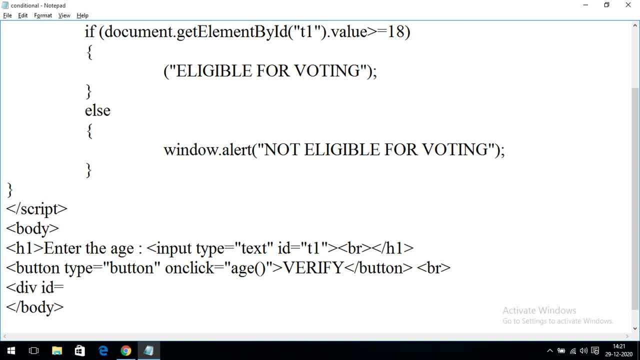 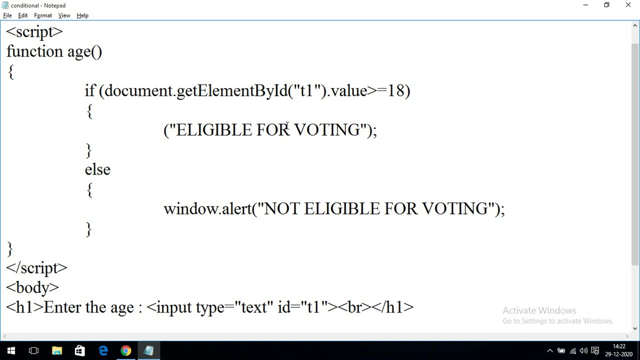 I will give some division tag. Give some ID is equal to some result. Close the division tag And here we can write. instead of writing all these things, we can write document dot. get element by ID of What is the result I think we have. 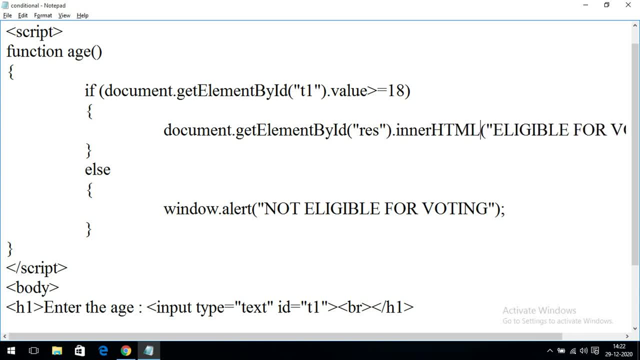 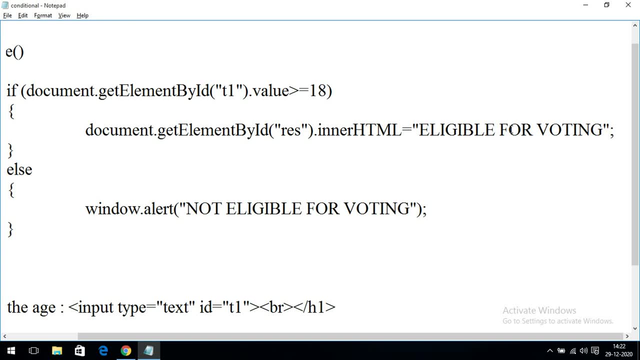 We have given some result. Dot inner HTML is equal to. So you can go with this one and close the. I mean remove the this one And just copy the same thing Here also, instead of using the windowalert. we can go with this one and remove the parentheses. 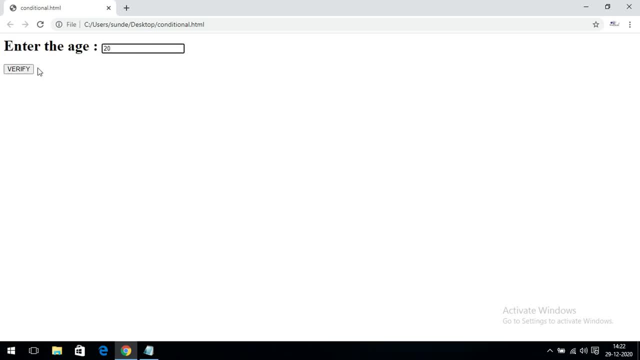 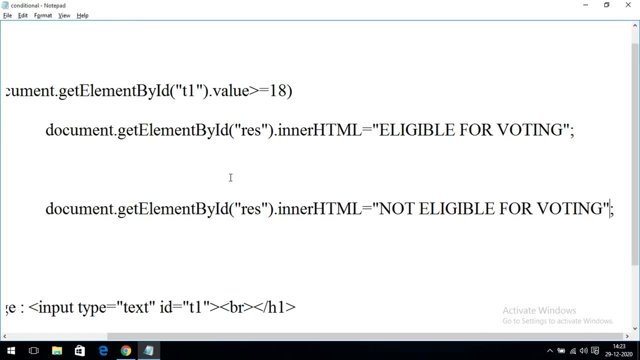 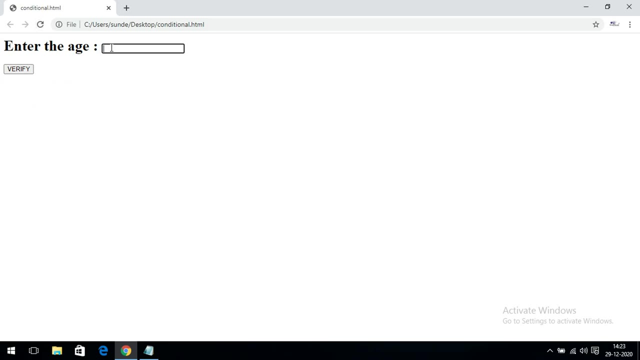 And you can observe here: enter the age, So 20.. We will get eligible for voting in this page itself. Okay, So we can use anything. We can use anything, Right, Say, not eligible for voting. And if you want to apply the some sort of styles for this one, you can simply go with the style tag. 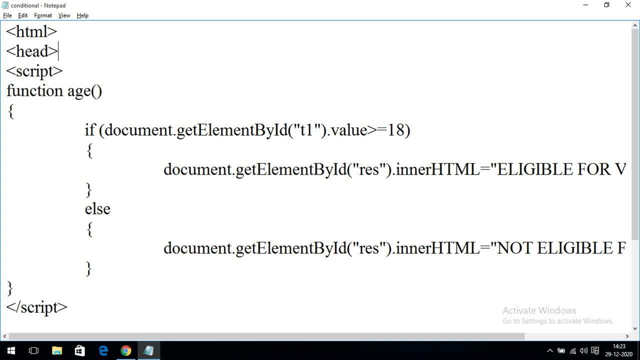 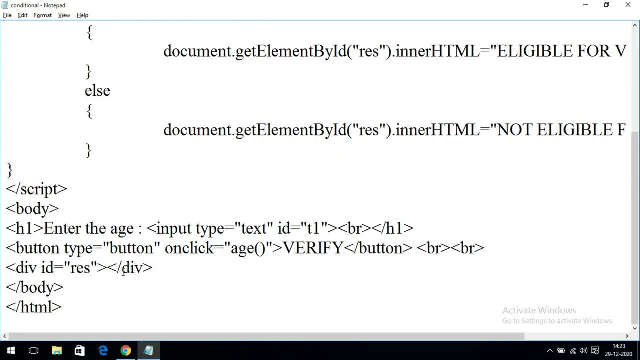 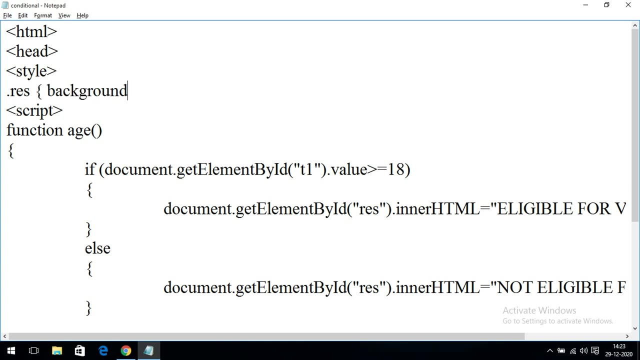 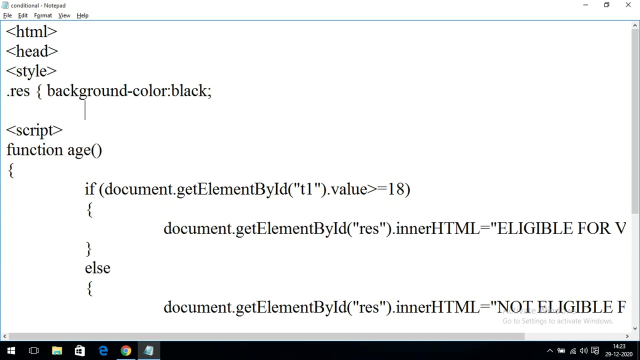 So inside the style, inside this one, go with the head tag and go with the style tag and see what is the idea of this one. result: so dot. a result is so: background color- some black and give some color. foreground color means font color, right, some white. 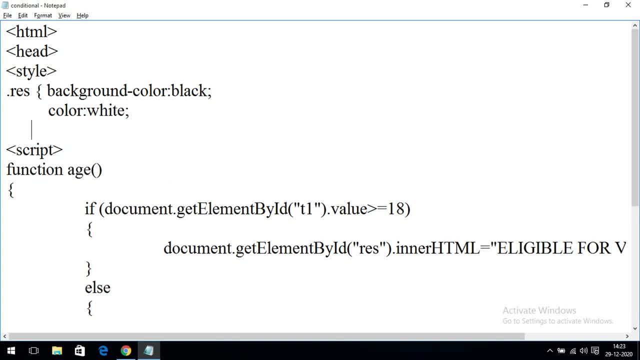 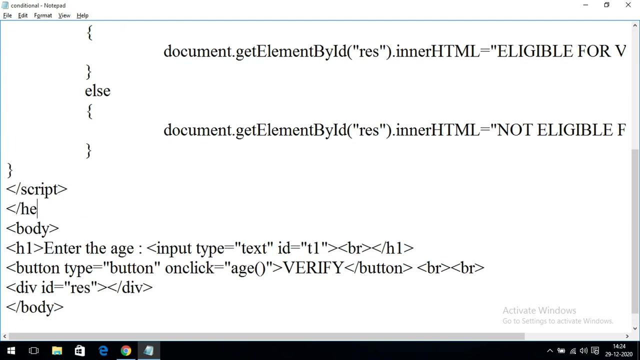 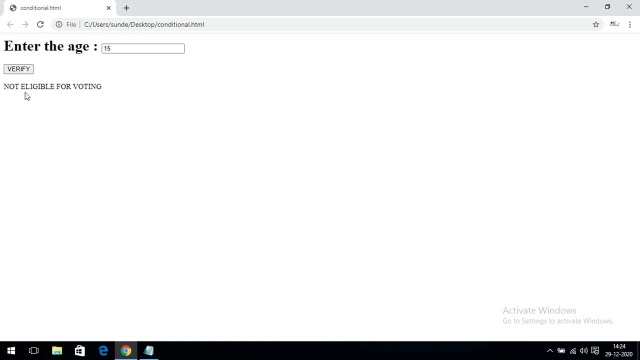 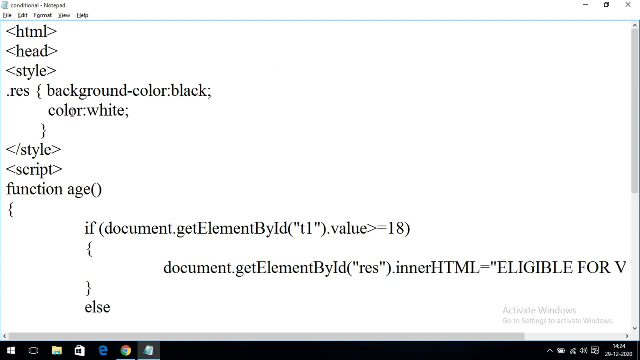 and also give some width. give some width, or else simply, you can close this one and we can check over that. see, I have to close the style tag and close the head tag. okay, now you can observe here. so if you go with the 15, we'll get, so not eligible for 14. yeah, here we have to go with the hash symbol. 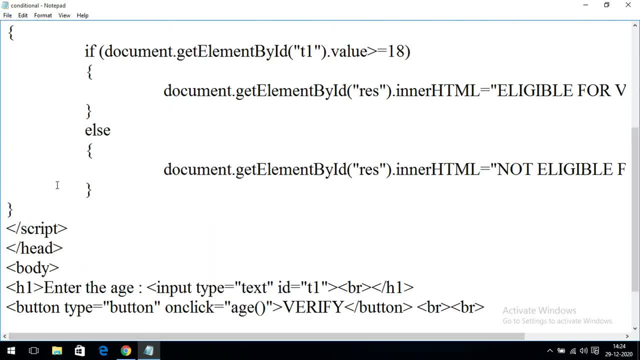 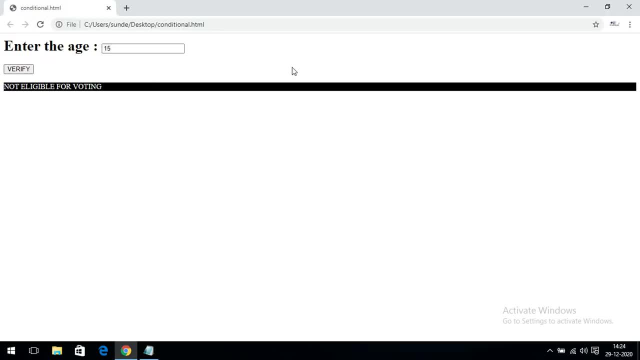 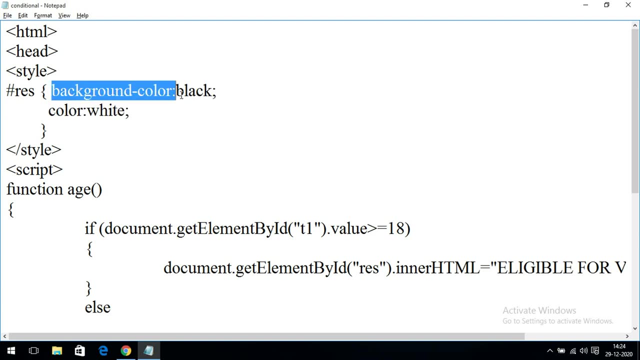 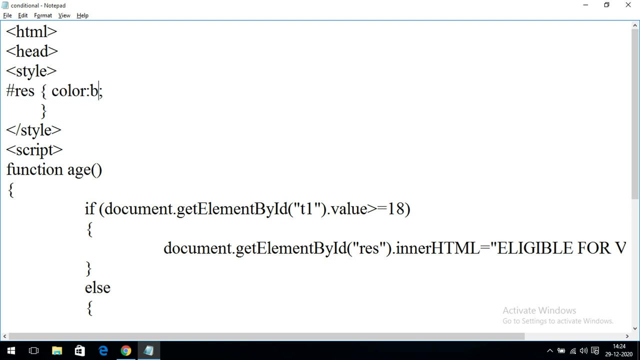 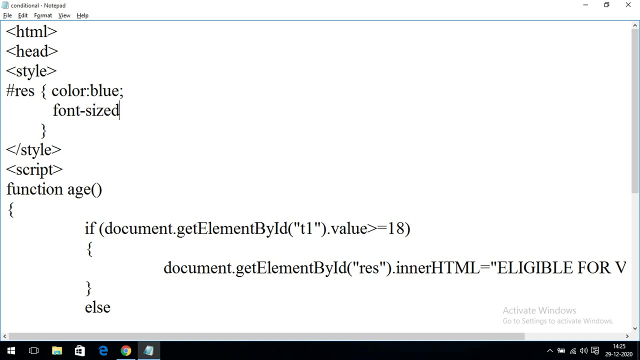 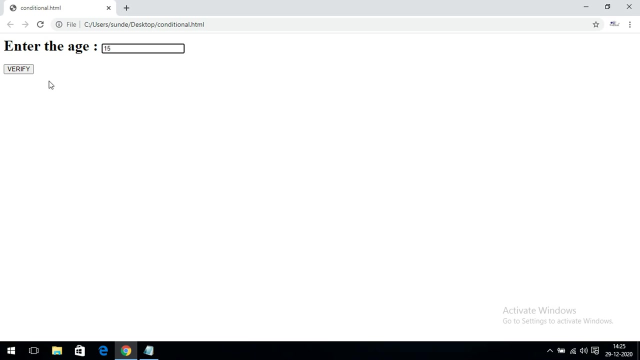 hash result. okay, because here we are using ID, so we have to use the hash symbol. you can observe. so background is black and foreground is white, right? so if you, if you remember this one, and simply use the color blue, font size- some 10 pixels- can check here: 15, enter right 30 pixels. you can move this one and simply use the color blue and font size- some 10 pixels. you can check here: 15, enter right 30 pixels. you can move this one and simply use the color blue and font size- some 10 pixels. you can check here: 15, enter right 30 pixels. you can move this one and simply use the color blue and font size- some 10 pixels. you can check here: 15, enter right 30 pixels. you can move this one and simply use the color blue and font size- some 10 pixels. you can check here: 15, enter right 30 pixels. you can move this one and simply use the color blue and font size- some 10 pixels. you can check here: 15, enter right 30 pixels. you can move this one and simply use the color blue and font size- some 10 pixels. you can check here: 15, enter right 30 pixels. you can move this one and simply use the color blue and font size: some 10 pixels. you can check here 15. enter right 30 pixels. you can move this one and simply use the color blue and font size: some 10 pixels you can check. 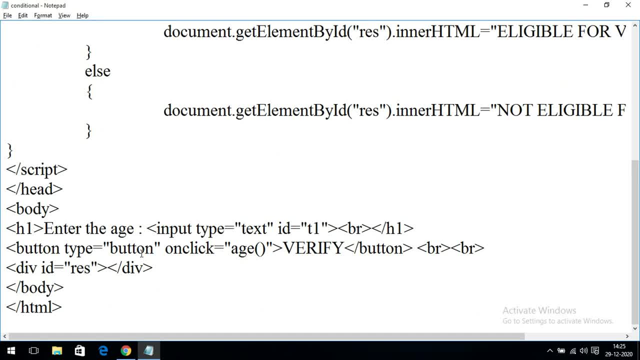 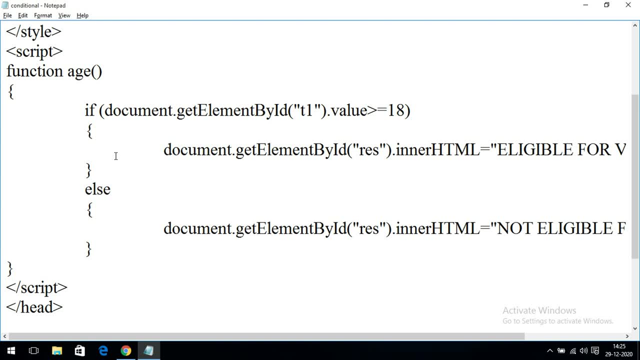 here: 15- enter right 30 pixels. you can move this one and simply use the color blue and font size- some 10 pixels. you can check here: 15- enter right 30 pixels. you can move this one and simply use the color blue and font size- some 10 pixels. you. 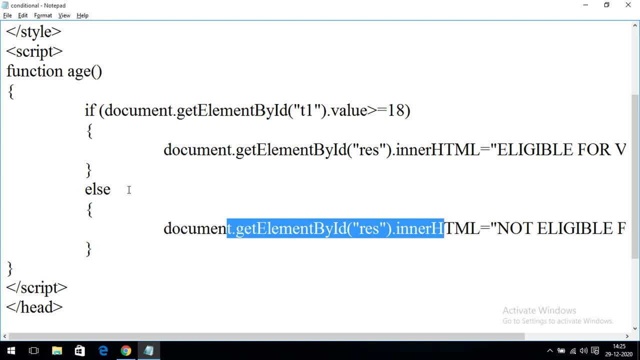 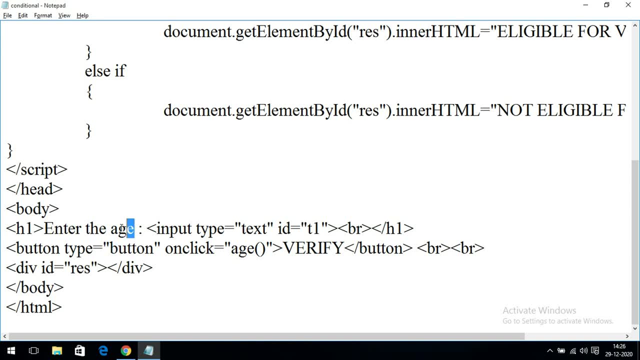 Once the condition is false again, if you want to check one more condition, then we have to use the else. if So, for that I will give you one more thing. See here we will write some: enter first number. and the same thing. we will write one more line: enter second number. 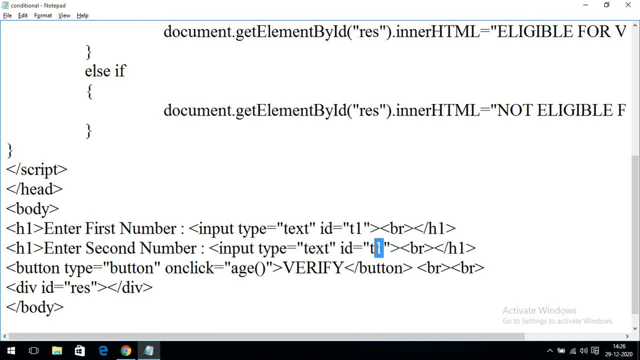 So we are taking some two numbers and we are finding the relation between those things. Okay, See, the same thing. I am not giving anything. So here I will write some relation, Relation. So here I will change relate two numbers. 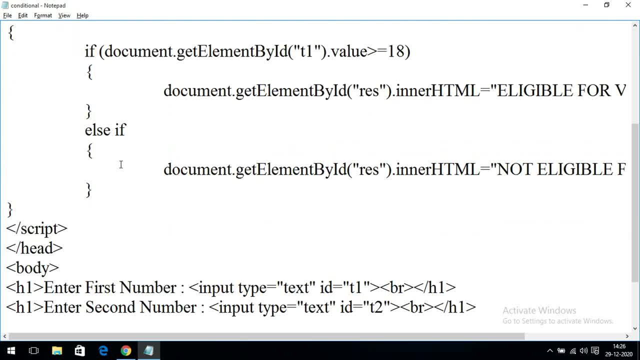 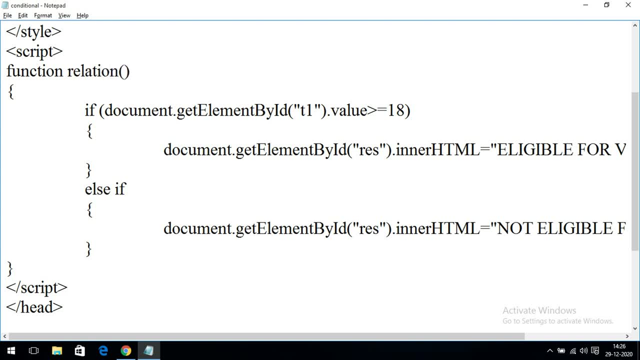 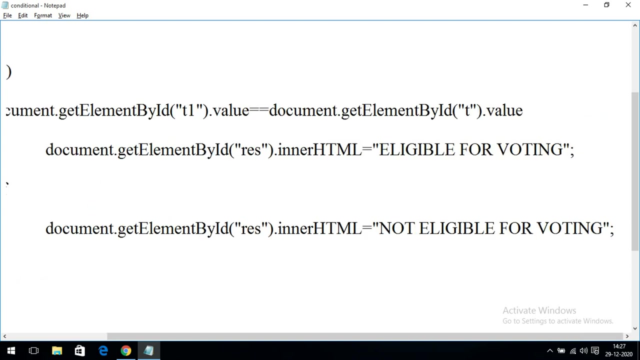 Relate two numbers and see I have to change the This one also. So this is a relation which we have done And here write down document: dot value: Same thing If both are equal: T2 dot value Right. Hope you understood this one. 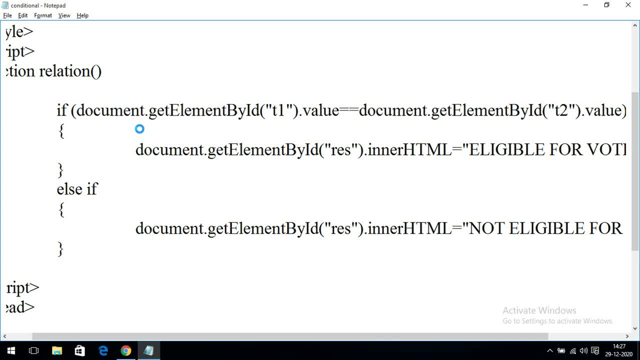 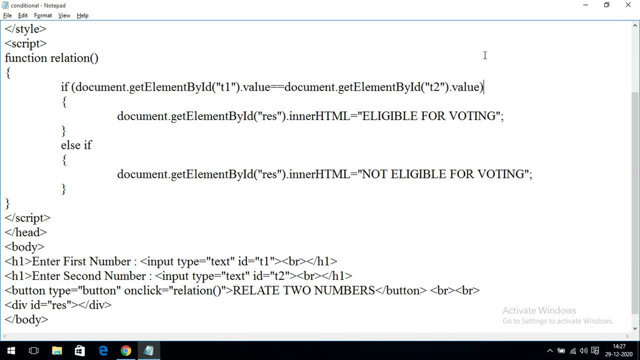 So I will decrease the font So that it will be readable, So I will go with 20.. Yeah, See, if both the values are equal, then you can write here: both are equal And else, if again if the condition is false, and copy the same thing here. 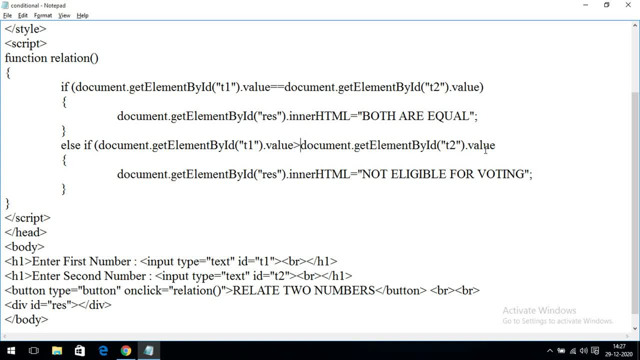 So it will be the same expression also that the second number, realtorarp, and then the second number. So if that condition is not great, then let's say half of 1 and then we beat this hell. First number And let's say first number. 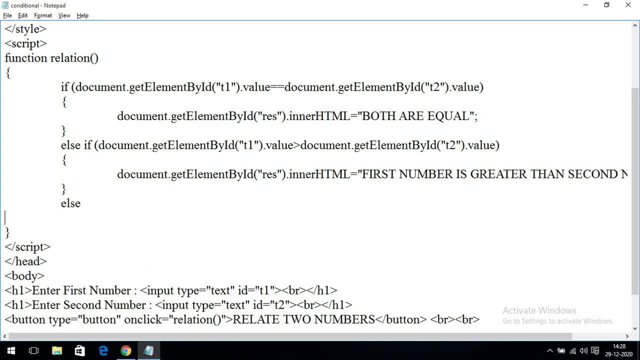 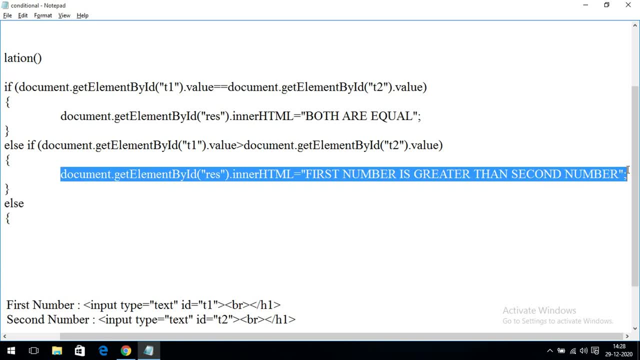 So let's say the first number we can remove, So it is a sentence. So I will write the second number into which, So we get it actually half. the second number is greater than first number, or we can simply write the first. 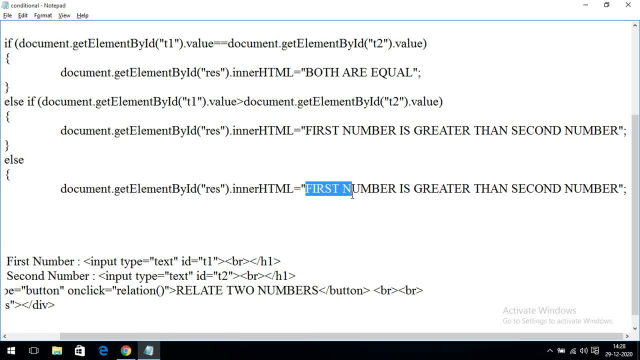 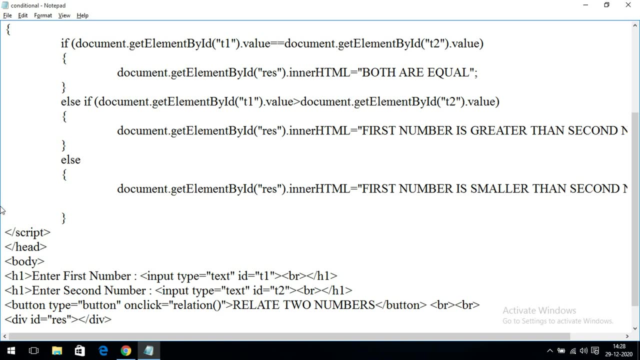 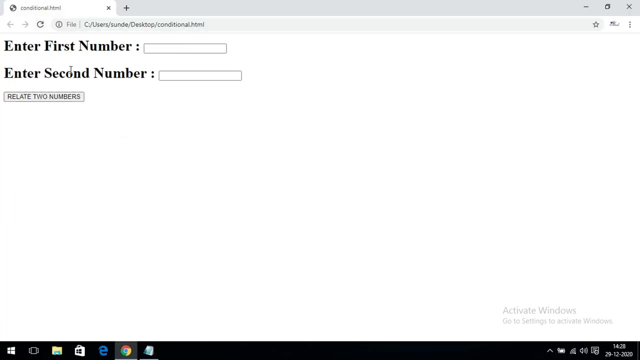 number is smaller than the second number, Instead of writing the greater smaller than the second number. ok, And yeah, you can observe here Now see: enter the first number, enter the second number. First number: I will enter 10,. second number: I will enter 20 and relate two numbers. So 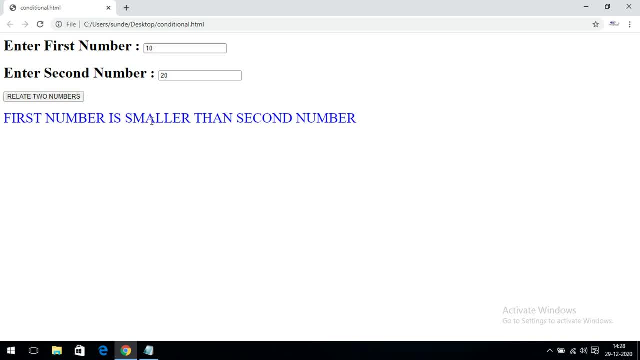 first number is smaller than the second number. So you can observe here 10 is smaller than 20 and you can simply go with this one, 10, relate two numbers and enter 10.. So we can see that here. So first number is greater than the second number and if you give both equal, if you relate, 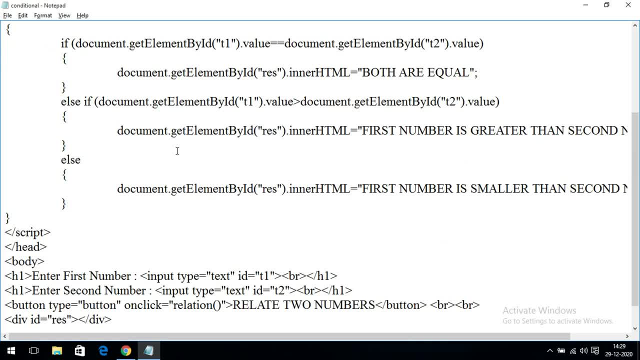 two numbers. both are equal. So like that, we can use the conditional statements, we can also use the conditional statements, right? So these are the conditional statements are simple: if, if else and else, if later. So if you are only verifying the true condition, then we will go with the simple if and if. 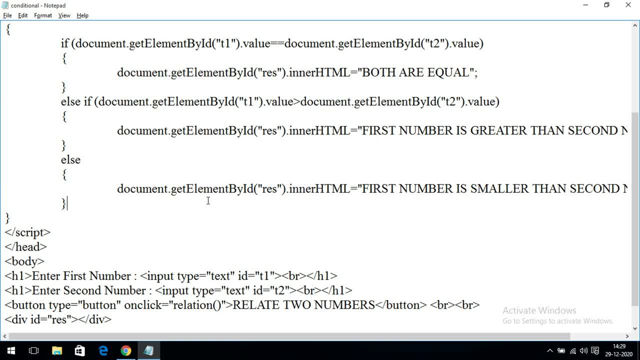 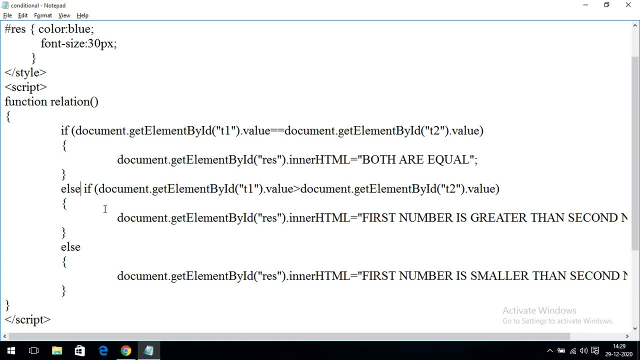 if you want to display both the true condition and a false condition, I mean, if you want to display either true condition or a false condition, then you can go with the if else right. Similarly, else if later, else if later. so we should not write any condition at the else. 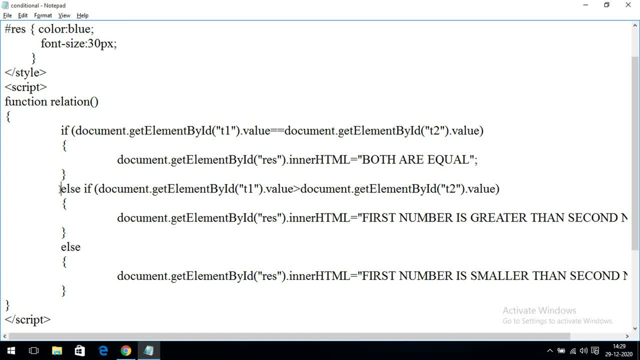 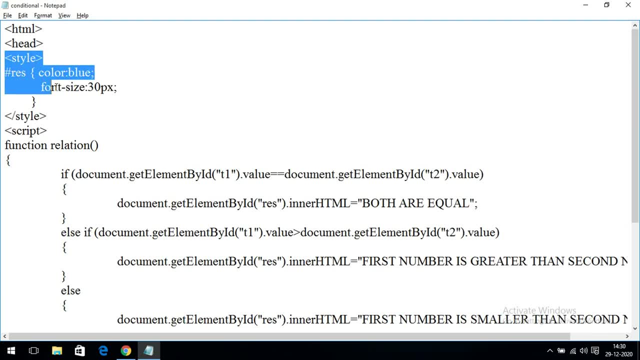 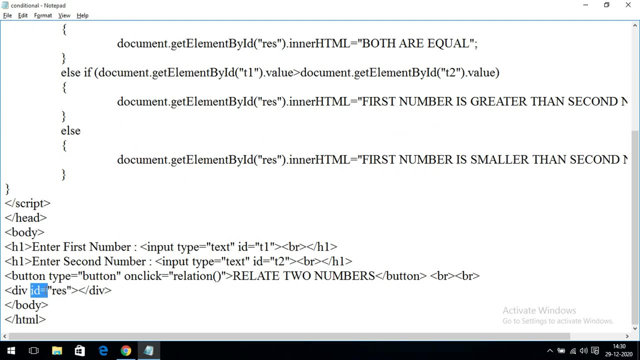 part. So if you want to write any condition in the else part, we have to use else. if you want to use else, if- and here we can also use the style sheets- and if you are not using the styles Normal, it will print it normal. so, based upon the id or class, we have to use the style. 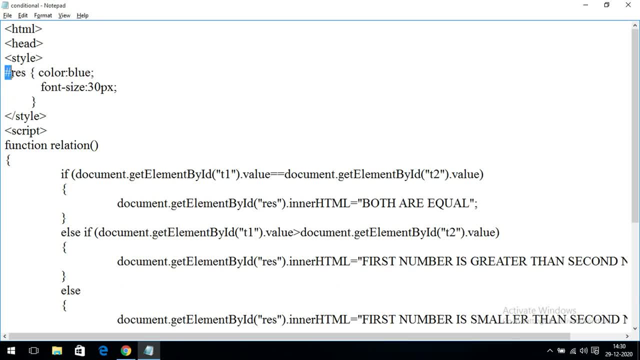 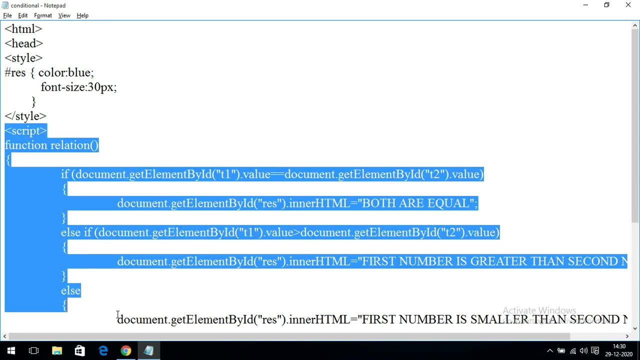 sheets. If you are using some id, we have to use hash symbol and if you are using some class, we have to use dot symbol, dot symbol and this styles should be written in between the styles style tag and that should be included in head and this script tag should be included in. 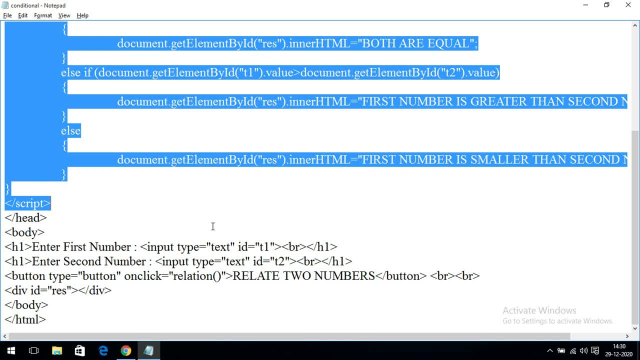 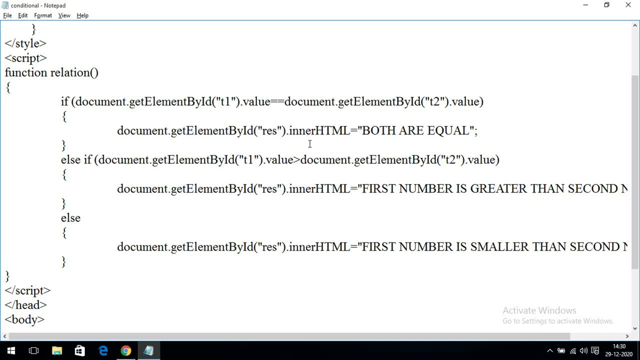 either head or body, so, which we have discussed earlier, And we can display the output by using one among the three output functions which we have discussed earlier, that is, innerHTML, dot, min, dot, writeln, or we can also go with the dot, I mean window, dot, alert, so we can go with the alert boxes, right? 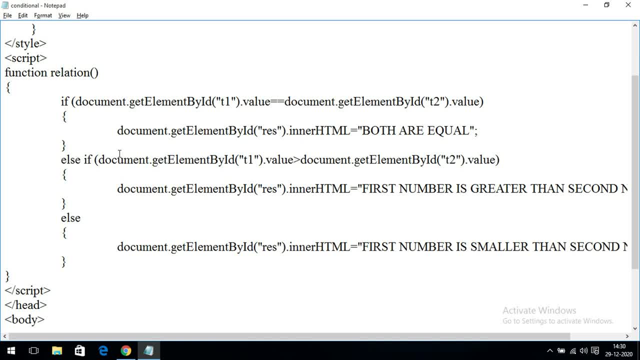 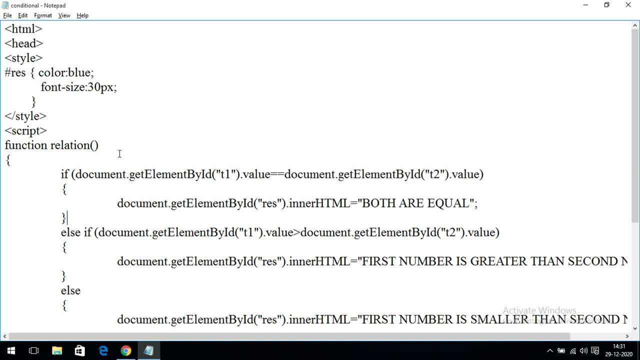 So hope you understood this: conditional statements. so if you are having any doubts regarding conditional statements, feel free to post your doubts in the comment section. Thank you So definitely. I will try to clarify all your doubts and if you really understood my session, like my session, share my session with your friends and don't forget to subscribe. to our channel. Thanks for watching. Thank you very much.